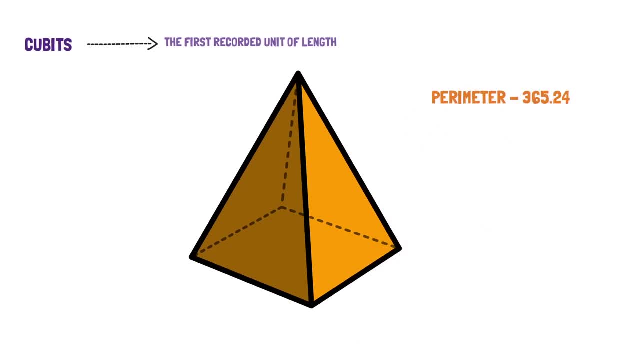 is 365.24, that is the number of days in the year. That the pyramid's perimeter divided by twice its height is equal to pi 3.1416.. Or that the king's chamber measurements are based on a Pythagorean triangle: 345.. 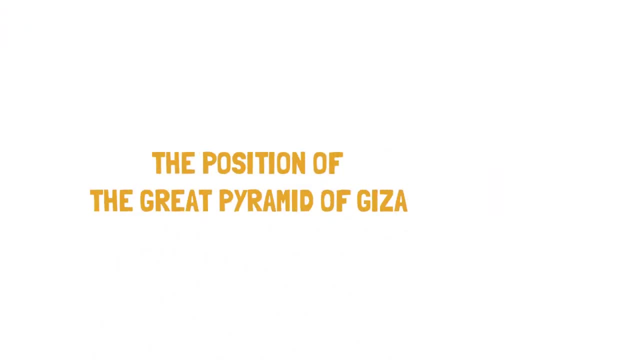 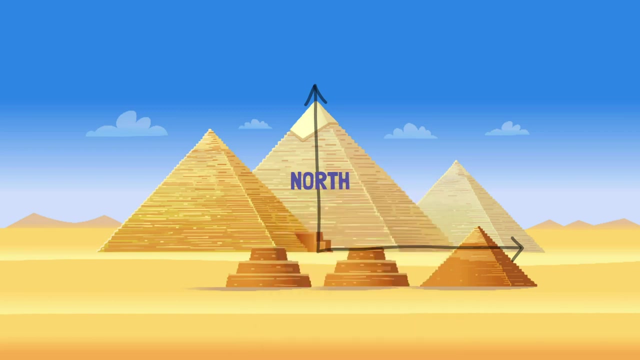 The Great Pyramid of Giza. The Great Pyramid is the most accurately aligned structure in existence and faces true north with only 3 x 60th of an degree of error. The position of the North Pole moves over time and the pyramid was exactly aligned at. 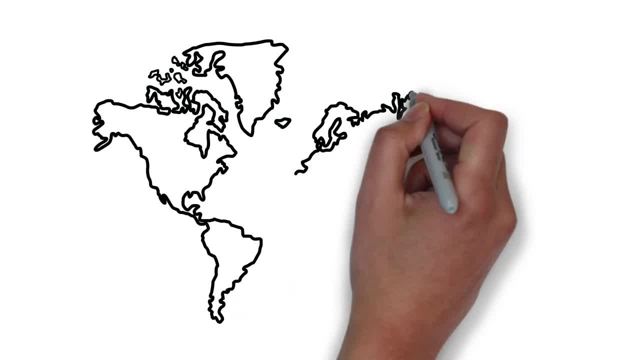 one time, But not only that. the Great Pyramid of Giza happens to be the center of Landmass. The Great Pyramid is located in the center of the Earth's formation. The Great Pyramid of Giza is located on the 읽iris, the corner of the Earth's axis. The Great Pyramid of 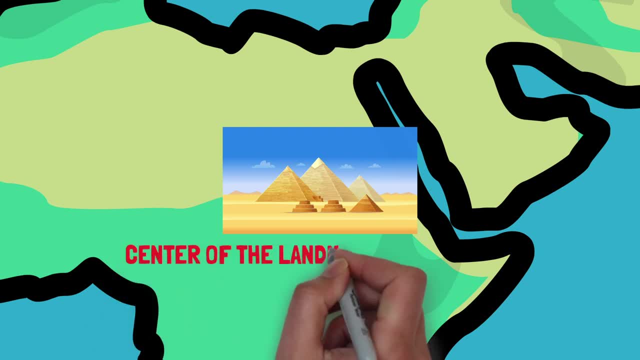 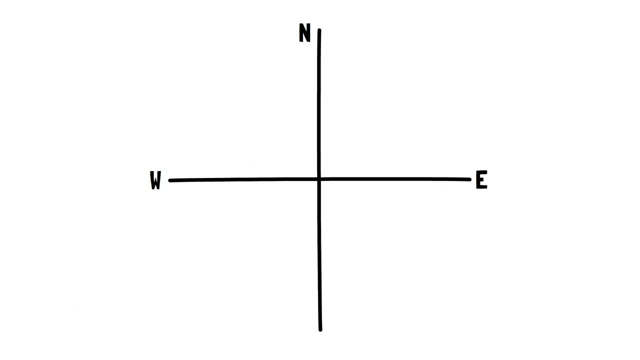 pyramid is located at the center of the landmass of the earth. The east or west parallel that crosses the most land and the north or south meridian that crosses the most land intersect in two places on the earth: one in the ocean and the other at the Great Pyramid. 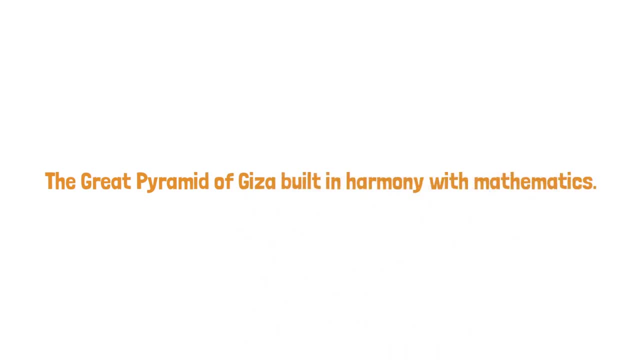 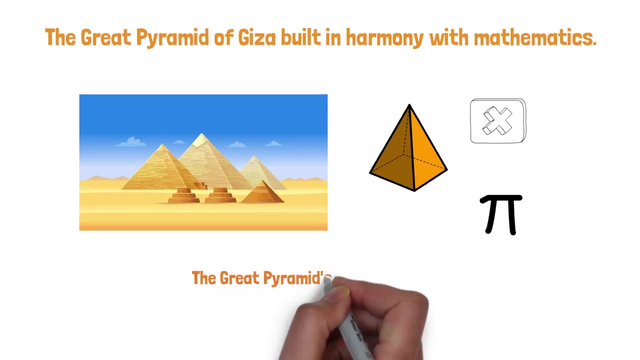 The Great Pyramid of Giza built in harmony with mathematics. Mathematically speaking, the Great Pyramid of Giza is perfect. The Great Pyramid's elevation encodes three of the most important constants in mathematics – pi, phi and e, According to detailed survey. 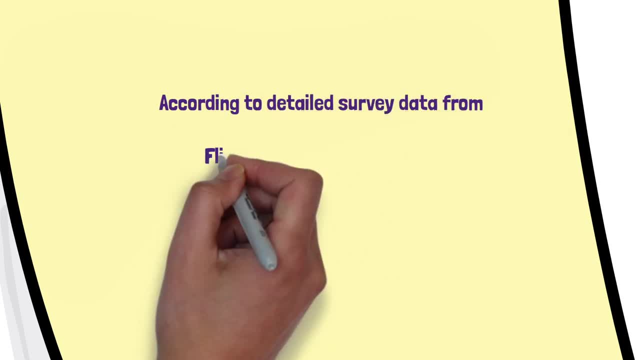 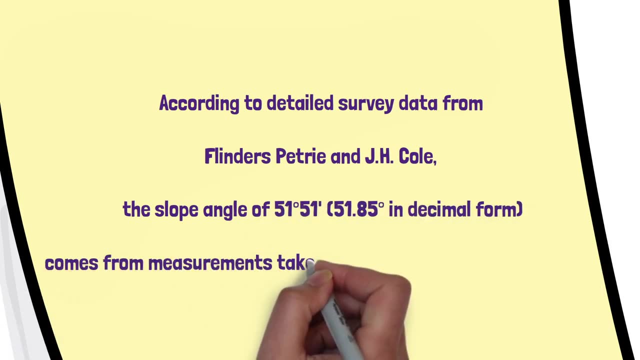 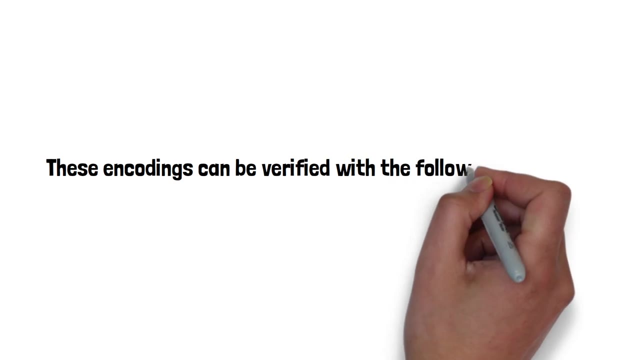 data from Flinders Petrie and J H Cole. the slope angle of 51.85° comes from measurements taken of the remaining casing stones. These encodes are the most important constants in mathematics. These encodes are the most Codings can be verified with the following equations: 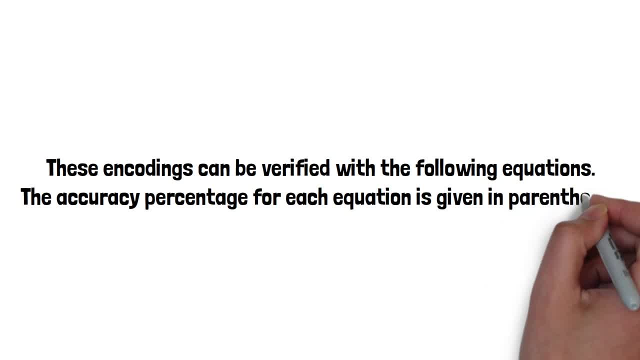 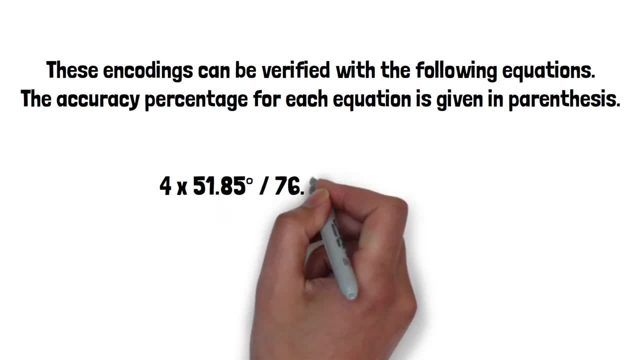 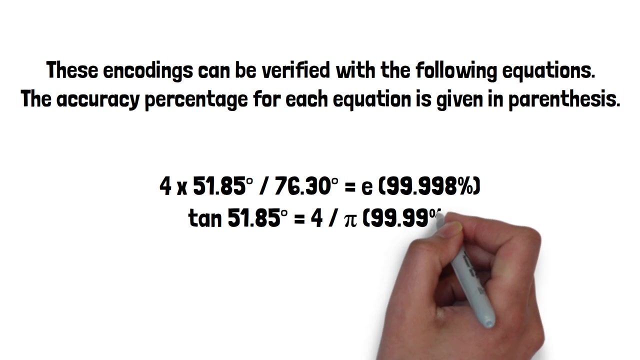 The accuracy percentage for each equation is given in parenthesis: 4 x 51.85° upon 76.30° is equal to E, which is 99.998%. Tan 51.85° is equal to 4 upon π, which is 99.99%. 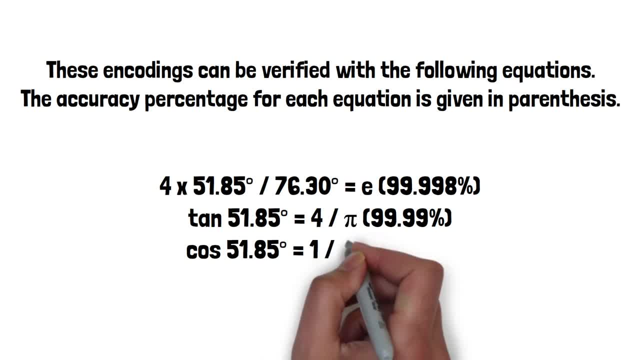 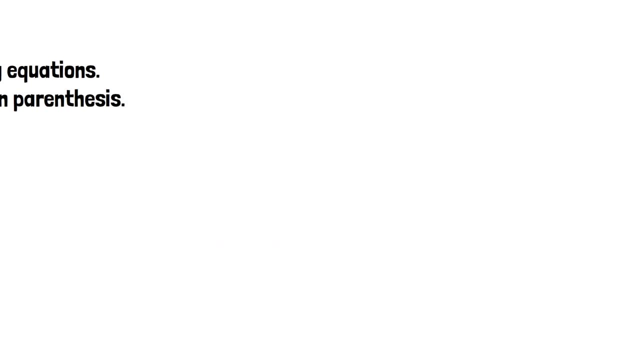 Cos 51.85 is equal to 1 upon 5, which is 99.95%, And sin 51.85° is equal to 4 upon π into 5, which is 99.94%. The constant e, known as Euler's number. 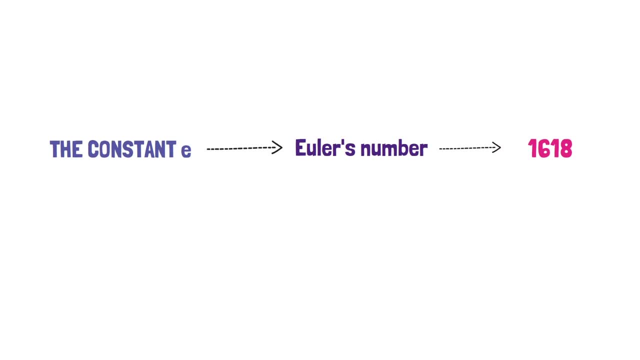 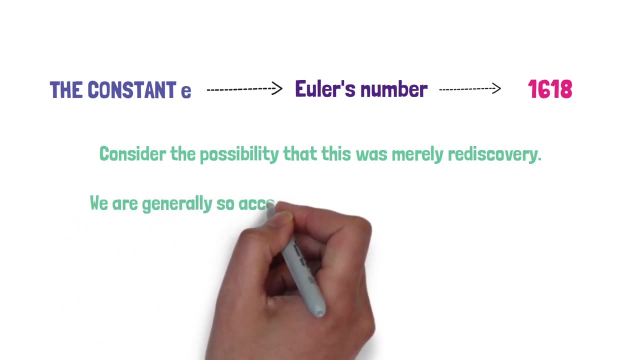 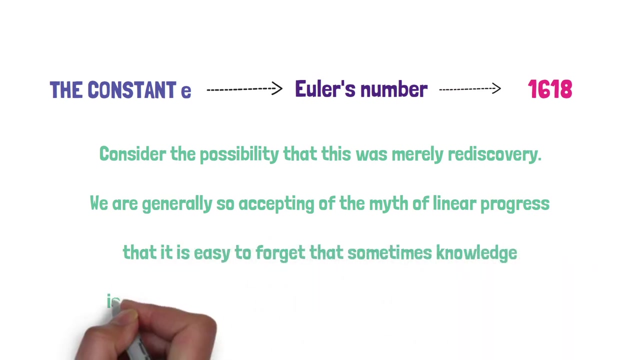 wasn't discovered until 1618.. Consider the possibility that this was merely rediscovery. We are generally so accepting of the myth of linear progress that it is easy to forget that sometimes knowledge is lost and not rediscovered for a very long time, if ever. The relationship 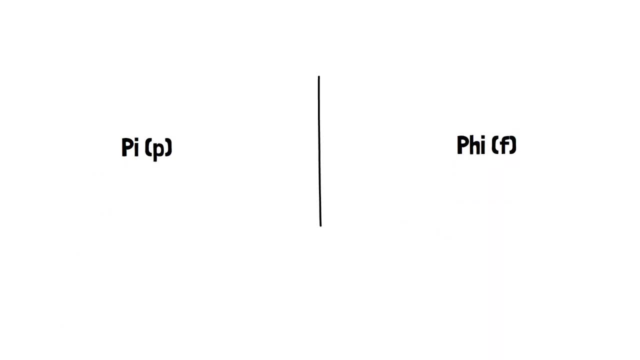 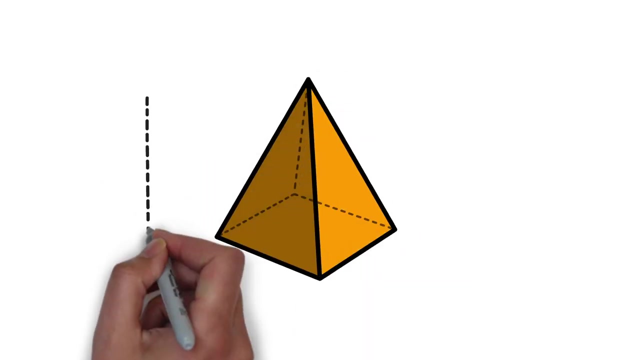 between pi and phi is expressed in the Great Pyramid's fundamental proportions. Pi is the relationship between the radius of a circle and its circumference. The mathematical formula is: circumference is equal to 2 into pi, into radius. The pyramid's vertical height holds the same relationship to the perimeter of its base, ie the distance around it. 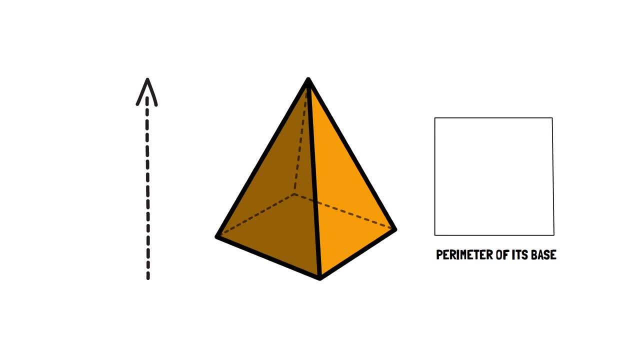 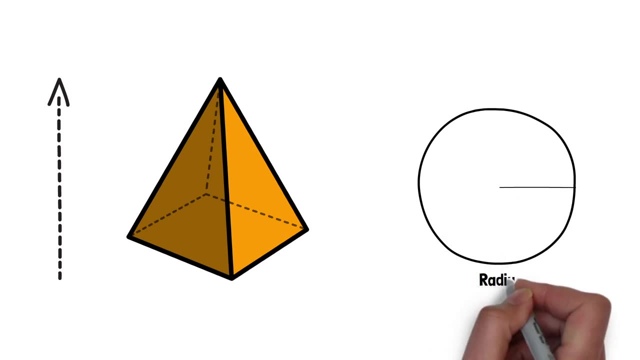 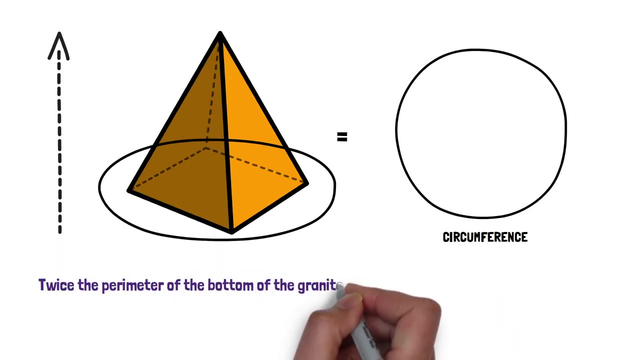 The radius of a circle bears due to its circumference. If we equate the pyramid's height to the radius of a circle, then the distance around the pyramid is equal to the circumference of that circle, Twice the perimeter of the bottom of the granite. coffer times: 10 power. 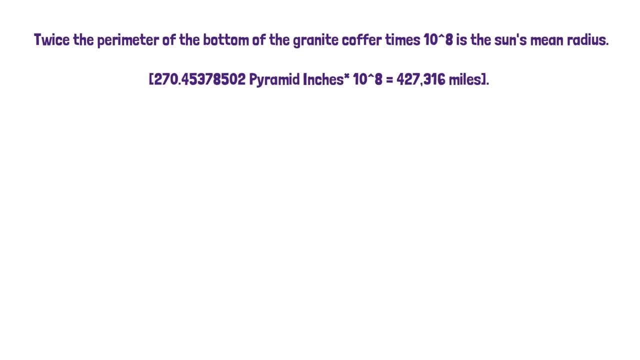 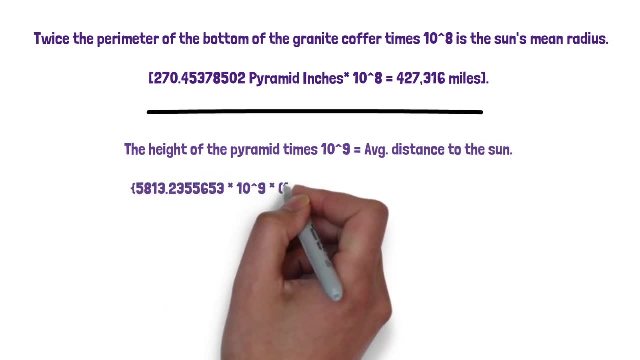 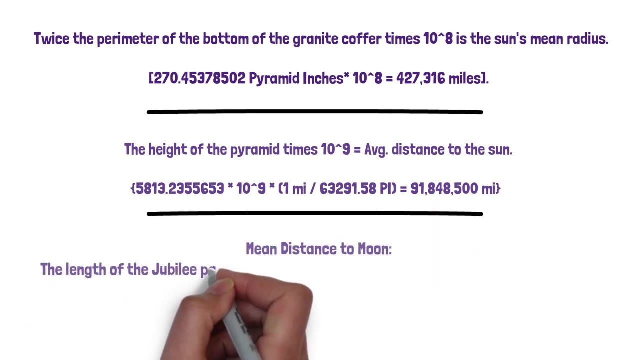 8 is the sun's mean radius. The height of the pyramid times 10 power 9 is equal to the average distance to the sun. Mean distance to the moon is the length of the jubilee passage times 7. times 10 power 7 is the mean distance to the moon. The weight of the pyramid is: estimated at 5,955,000 tons, Multiplied by 10 power 8 gives a reasonable estimate of the earth's mass. The sacred cube at times. 10 power 7 is equal to the polar radius of the earth. The curvature designed into the faces of the pyramid exactly matches the radius of the earth And, interestingly, 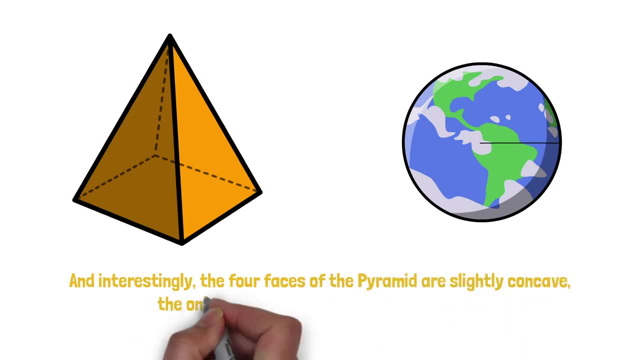 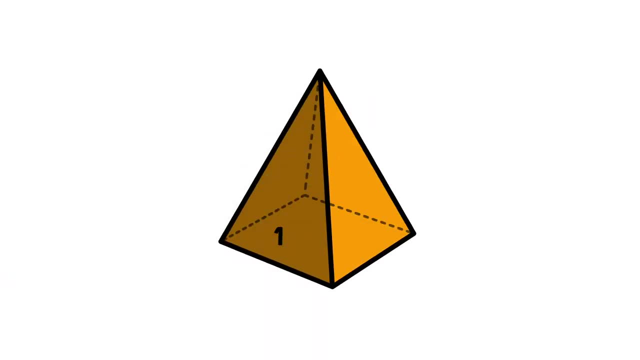 the four faces of the pyramid are slightly concave, the only pyramid to have been built this way. While most pyramids we see have four sides, the Great Pyramid of Giza is the only pyramid to have four sides, At dawn and sunrise, on the spring and autumn equinoxes. 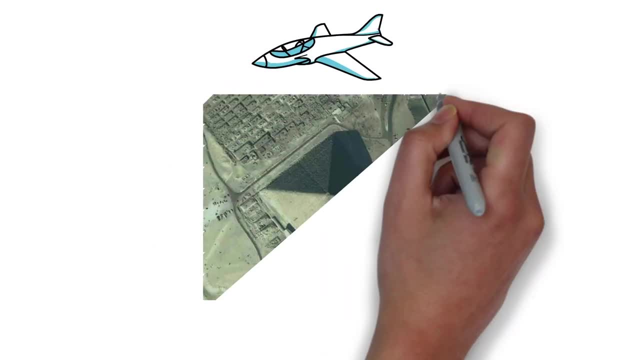 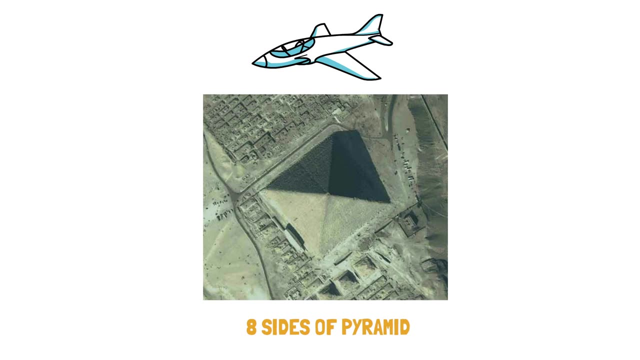 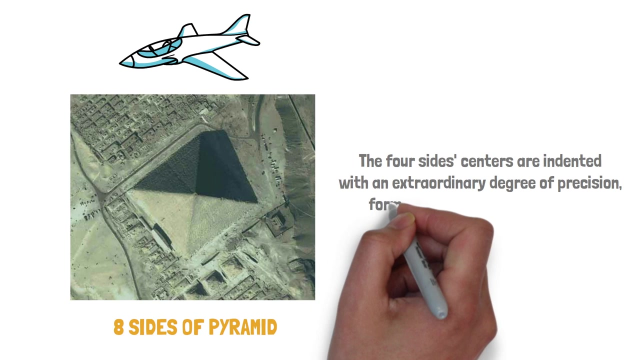 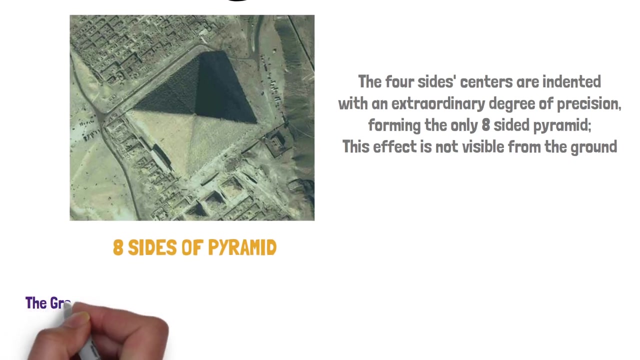 a phenomena only visible from the air reveals the eight sides of the pyramid. when the sun casts shadow on the ancient structure, The four sides' centers are intended, with an extraordinary degree of precision, forming the only eight-sided pyramid. This effect is not visible from the ground. The Great Pyramid of Giza is the only pyramid discovered. 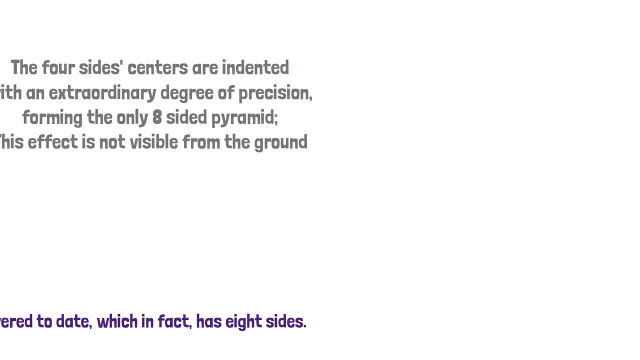 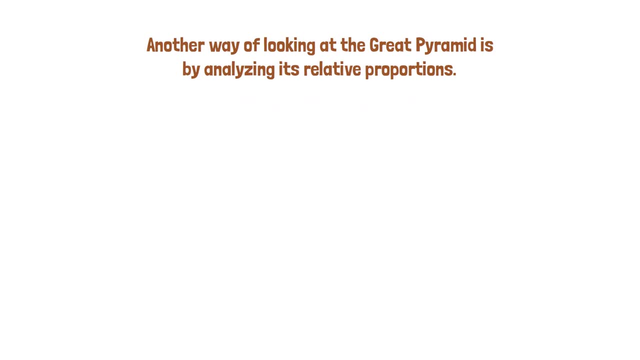 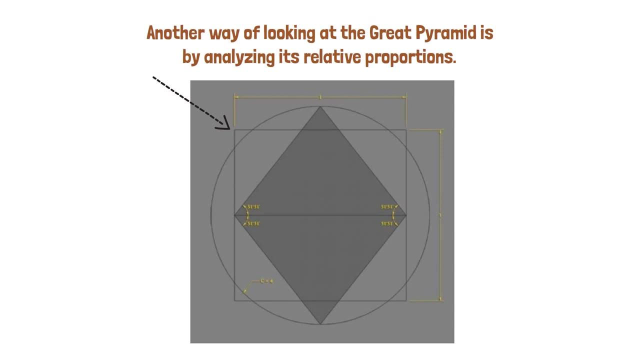 to date, which in fact has eight sides. Another way of looking at the Great Pyramid is by analyzing its relative proportions. If the base measures unit length, then a square with an equal unit edge can be drawn as shown below. A circle drawn from the center with radius of 1.8 meters can be drawn from the. 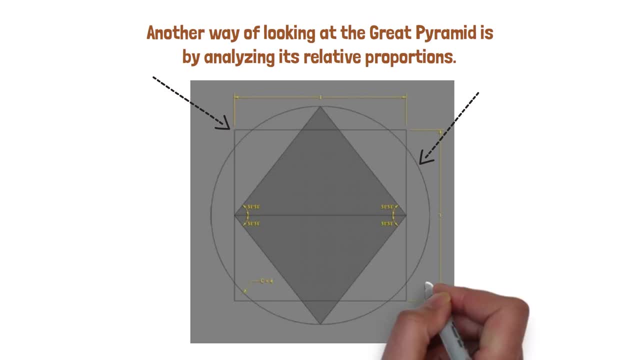 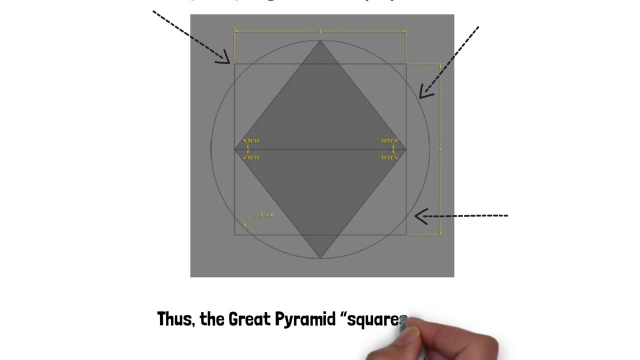 center. with radius of 1.8 meters. The pyramid of Giza can be easily measured With the. with radius equal to the height of the pyramid, has circumference equal to the square's perimeter. Thus the Great Pyramid squares the circle. Its form approximates the solution. 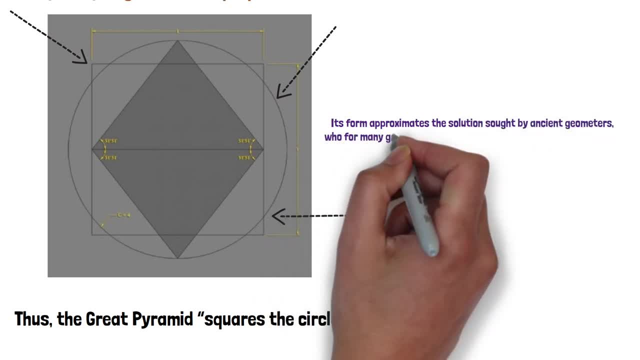 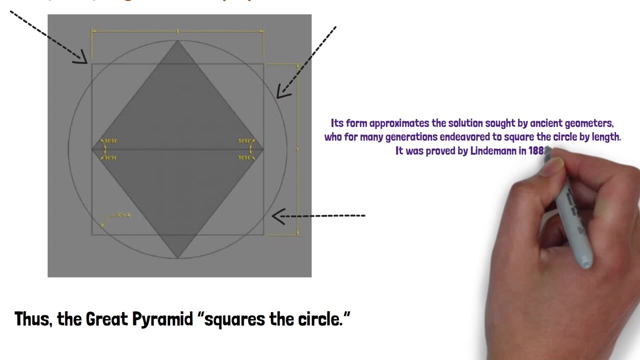 sought by ancient geometers who for many generations endeavoured to square the circle by length. It was proven by Lindemann in 1882,. exact squaring of the circle is impossible due to the transcendental qualities of pi, In addition to relative proportions when its elevation. 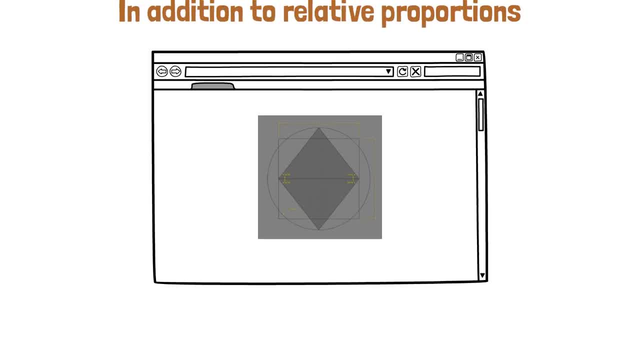 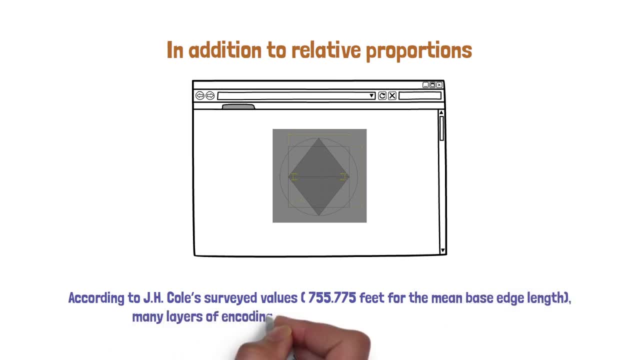 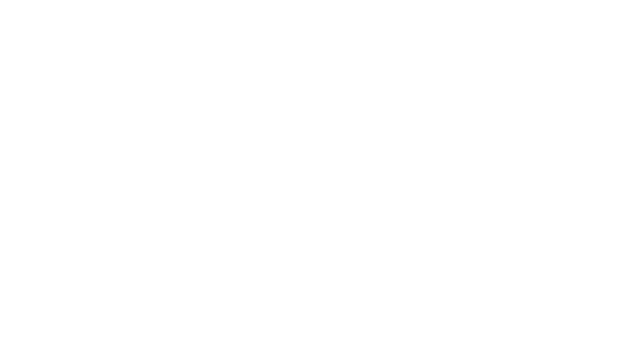 is drawn in a computer-aided design program in actual size. according to J H Cowell's surveyed values, many layers of encoding were rediscovered in the Great Pyramid by taking its precise and precise measurements. For example, if an equilateral triangle is inscribed inside, this is what immediately 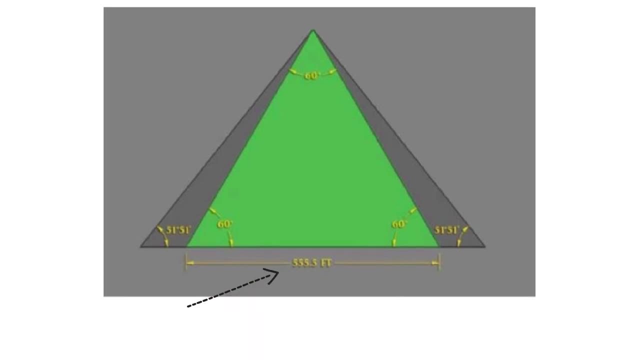 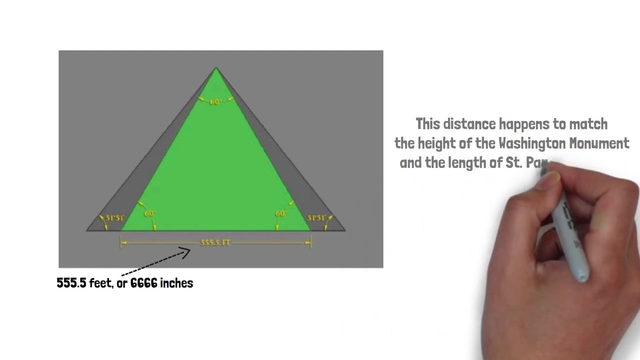 pops out, The green triangle's edge length is 555.5 feet or 6,666 inches. This distance happens to match the height of the Washington Monument and the length of St Paul's Cathedral, And the same goes for in111.2 inches, but the key pattern to observe is repeating digits. 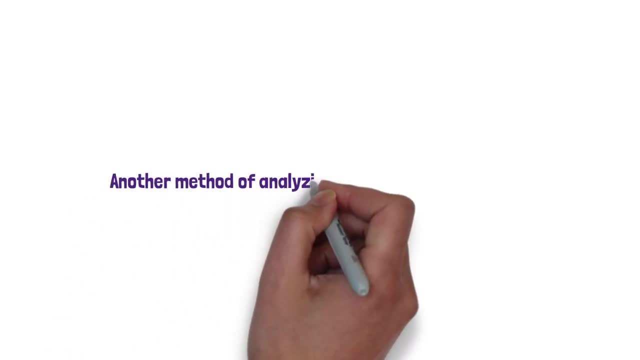 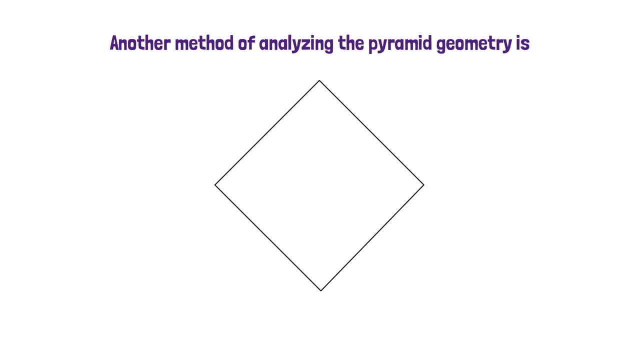 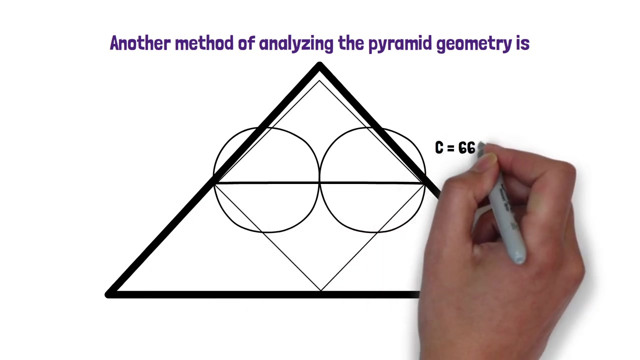 Another method of analysing the pyramids' symmetry is with a square rotated 45° with respect to ground plane. The largest square that fits inside the pyramid's elevation encodes 2 circles across its diagonals having circumferences equaling exactly 666.6 ft each. Only so each square slightly more 이�. 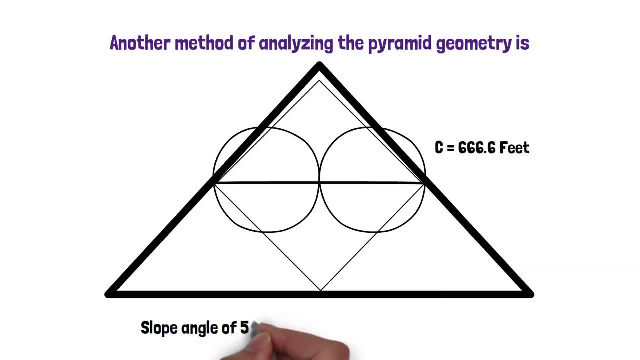 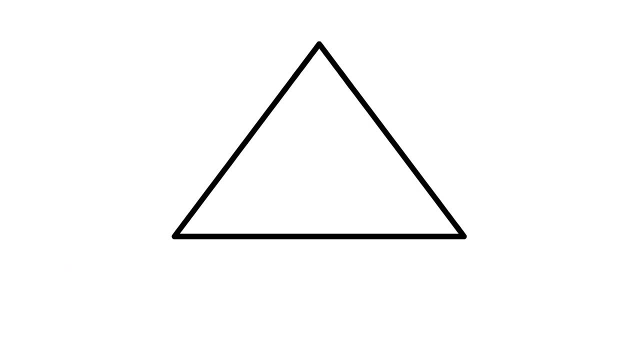 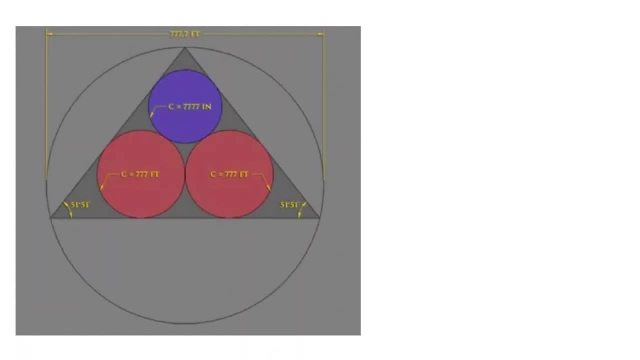 each allowing that the slope angle of 51 degree 51 inches has an accuracy of only 99.8%. If you circumscribe the pyramid's elevation triangle and then measure the circle's diameter, this equals 777.7 feet, ie 99.97% accurate with a slope of 51 degree 51 inches and base. 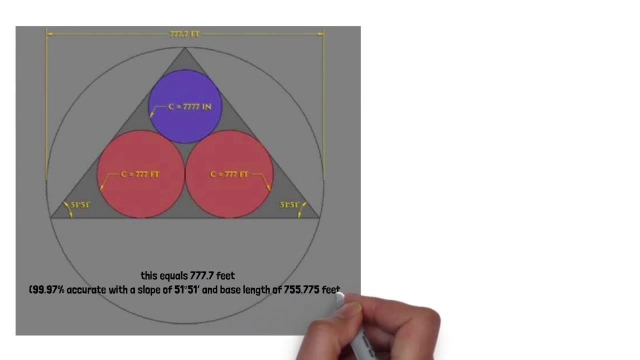 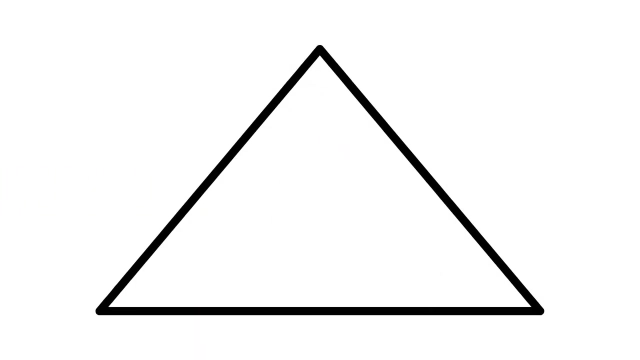 length of 755.775 feet. In addition, the inscribed circles shown below in red and blue have circumferences of 777 feet and 7777 feet Sevens abound. This next image depicts a single inscribed circle having a diameter of 365.242 feet inside. 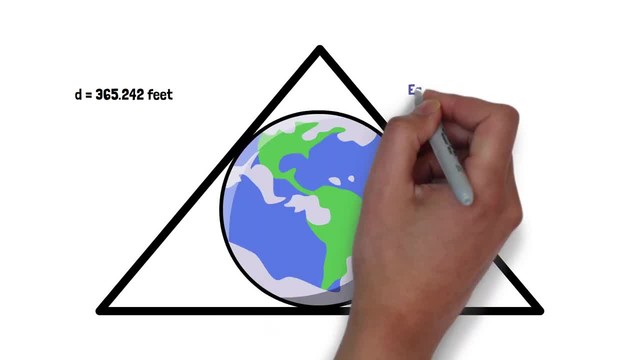 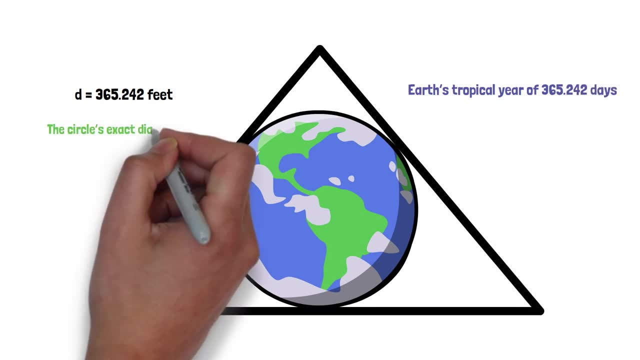 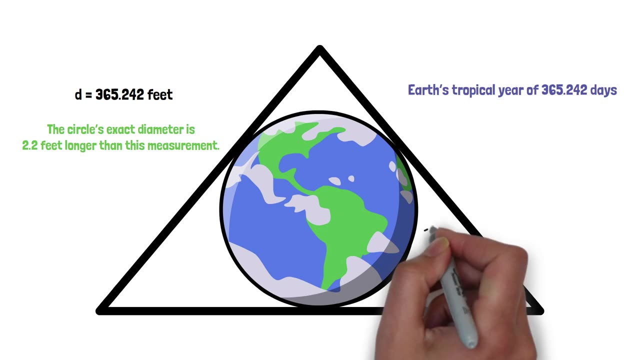 the pyramid's elevation that echoes Earth's tropical year of 365.242 days. The circle's exact diameter is 2.2 feet longer than this measurement, But the small delta might reference the Earth's atmosphere, which is like an onion's skin. 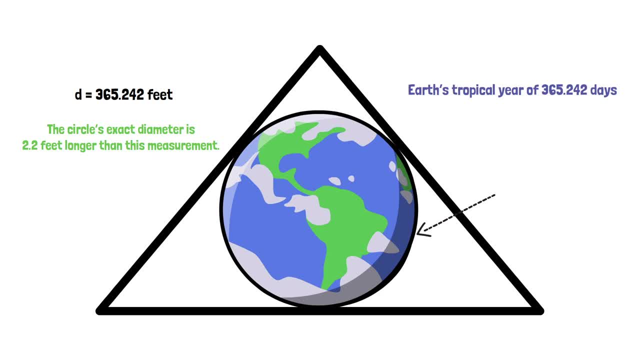 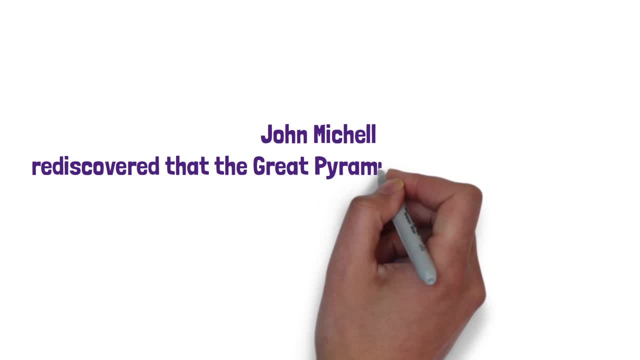 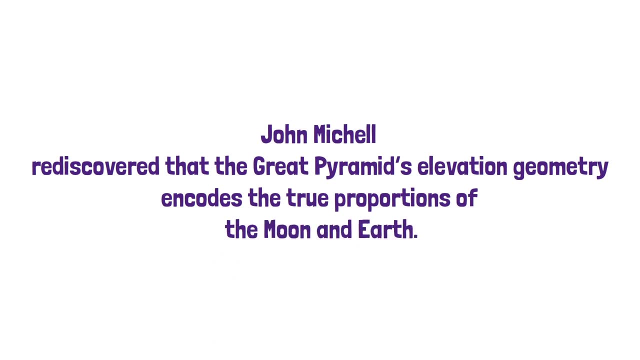 at this scale, roughly equalling the thickness of the diagram's lines. Writer and deep thinker John Mischel rediscovered that the Great Pyramid's elevation geometry encodes the true proportions of the Moon and the Earth. This is evident when you bring these two bodies together. 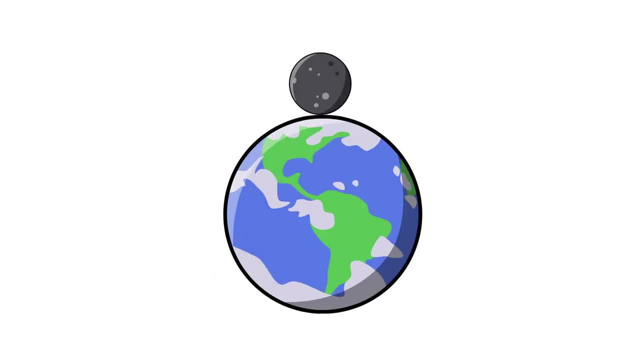 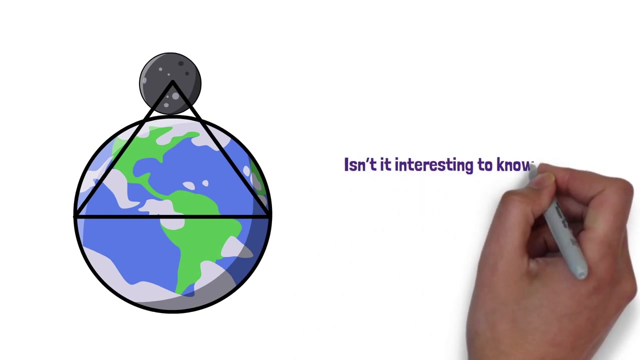 Such that they are equal, Such that the Moon is tangent to Earth's surface. The tip of the shaded pyramid diagrammed below is at the centre of the Moon, and the base of the pyramid runs along Earth's equator. Isn't it interesting to know the mathematics concept associated with these historic pyramids?